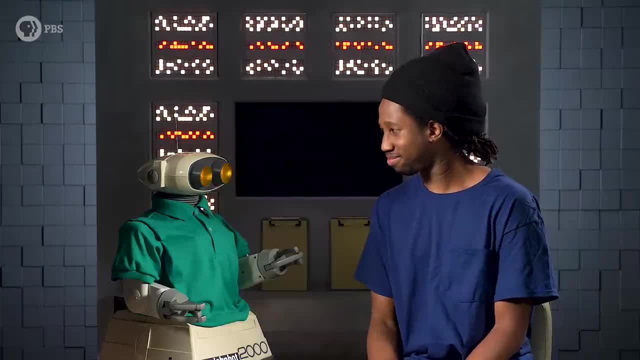 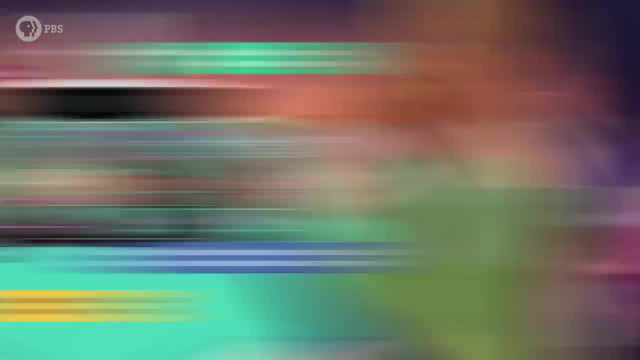 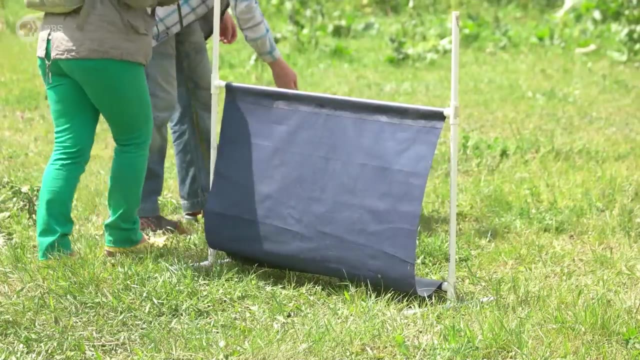 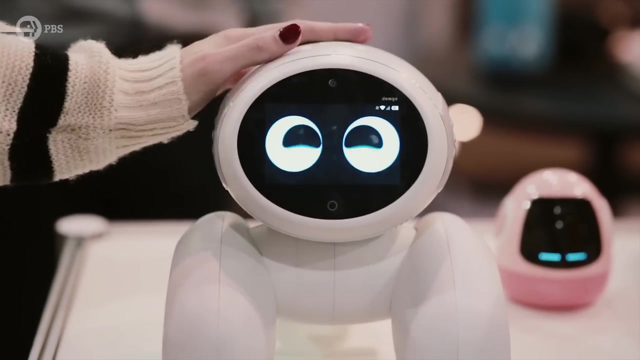 called supervised learning. You ready, John Greenbot? Hello, humanoid friend, The process of learning is how anything can make decisions, Like, for example, humans, animals or AI. They can adapt their behavior based on their experiences. In Crash Course AI, we'll talk about three main types of learning: Reinforcement, unsupervised. 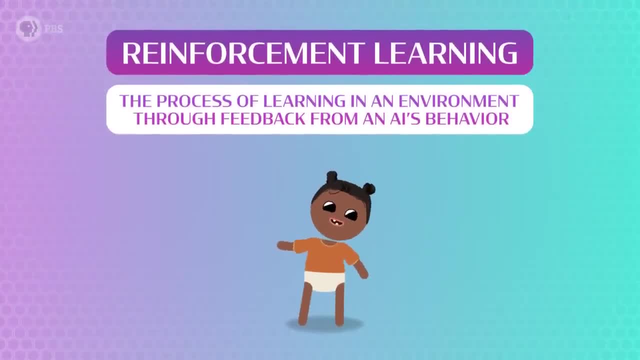 and supervised learning. Reinforcement learning is the process of learning in an environment through feedback from an AI's behavior. It's how kids learn to walk. No one tells them how. they just practice, stumble and get better at balancing until they can put one foot in front of the other. 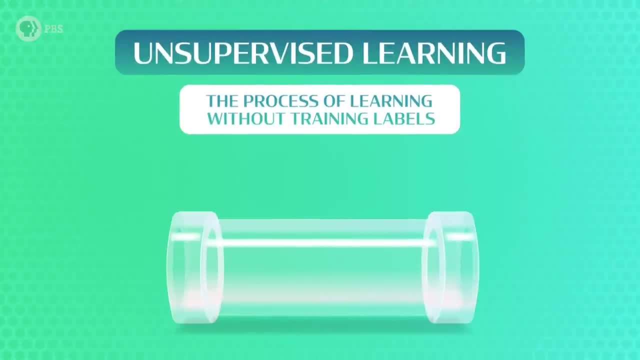 Unsupervised learning is the process of learning without training labels. It could also be called clustering or grouping. Sites like YouTube use unsupervised learning to find patterns and frames of video and compress those frames so that videos can be streamed to us quickly. 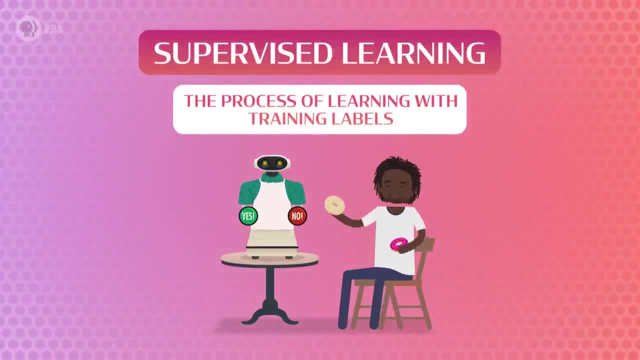 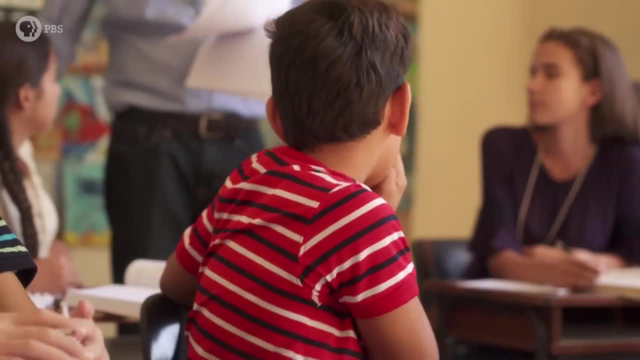 And supervised learning is the process of learning with training labels. It's the most widely used kind of learning when it comes to AI and it's what we'll focus on today and in the next few videos. Supervised learning is when someone who knows the right answer called a supervisor points. 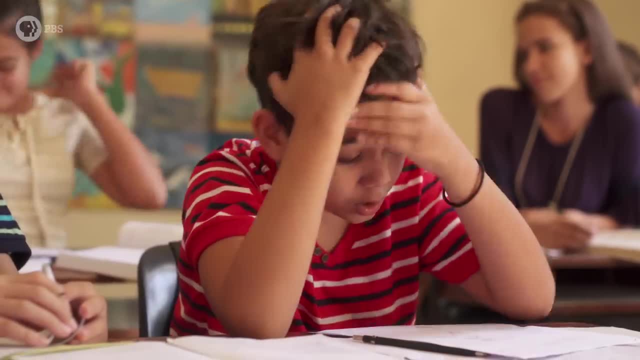 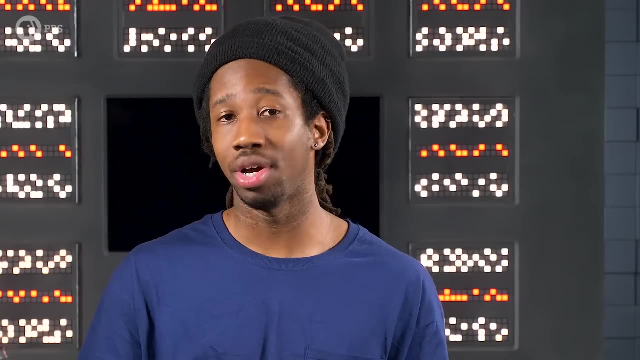 out mistakes during the learning process. You can think of this like when a teacher corrects a student's math In one kind of supervised setting. we want an AI to consider some data, like an image of an animal, and classify it with a label like reptile or mammal. 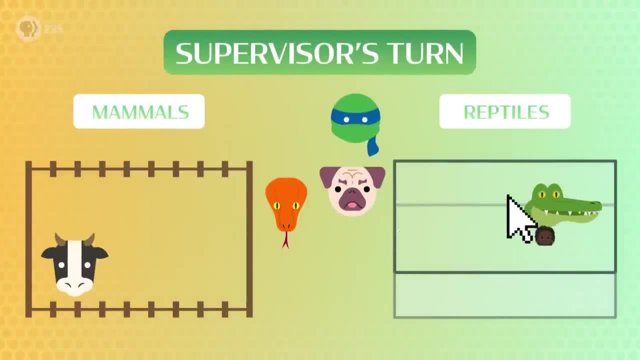 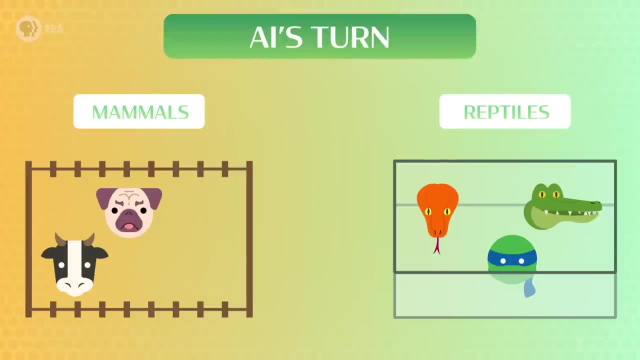 AI needs computing power and data to learn, and that's especially true for supervised learning, which needs a lot of training examples from a supervisor. After training this hypothetical AI, it should be able to correctly classify images it hasn't seen before, like a picture of a kitten as a mammal. That's how we know it's learning. 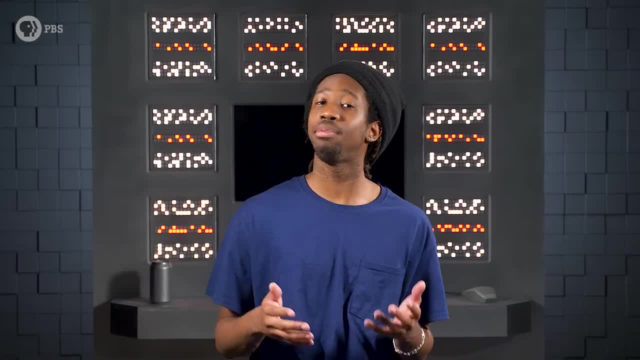 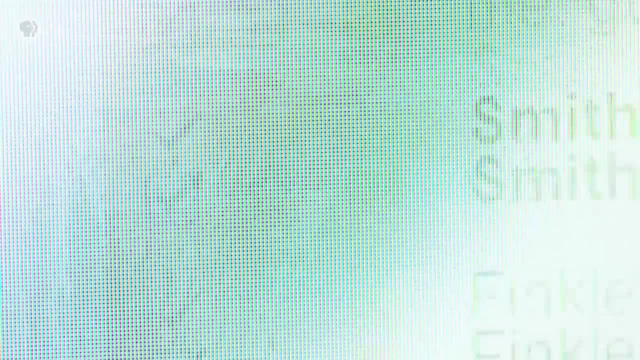 instead of just memorizing answers, And supervised learning is a key part of lots of AI you interact with every day. It's how email accounts can correctly classify a message from your boss as important and ads as spam. It's how Facebook tells your face apart from your friend's face, so that it can. 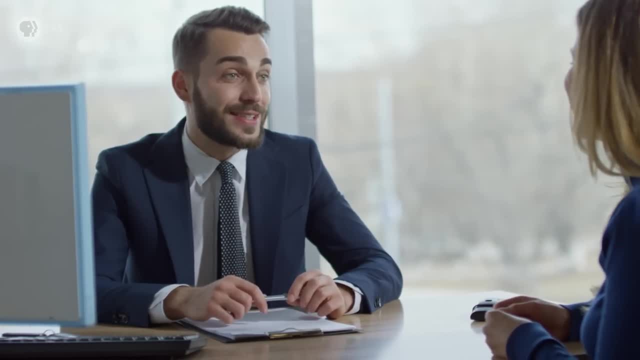 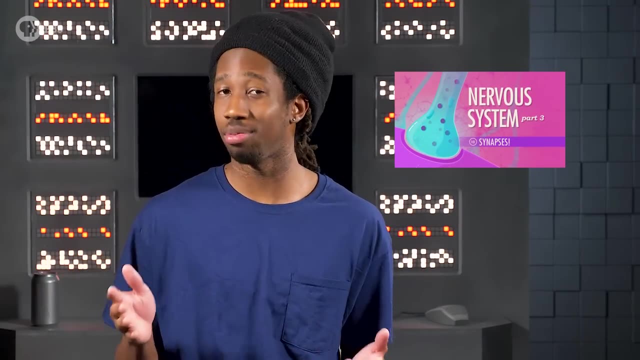 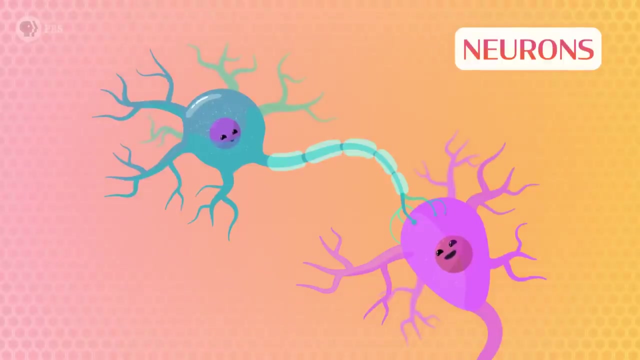 make tag suggestions when you upload a photo And it's how your bank may decide whether your loan request is approved or not. Now, to initially create this kind of AI, computer scientists were loosely inspired by human brains. Human brains have billions of them. Each neuron has three basic parts: the cell body. 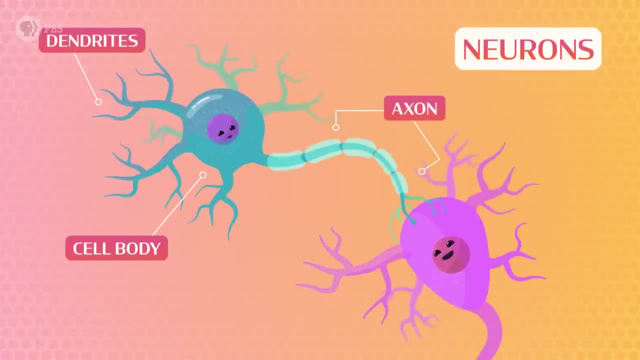 the dendrites and the axon. The axon of one neuron is separated from the dendrites of another neuron by a small gap called a synapse, and neurons talk to each other by passing electric signals through synapses. As one neuron receives signals from another neuron, the electric energy inside of its 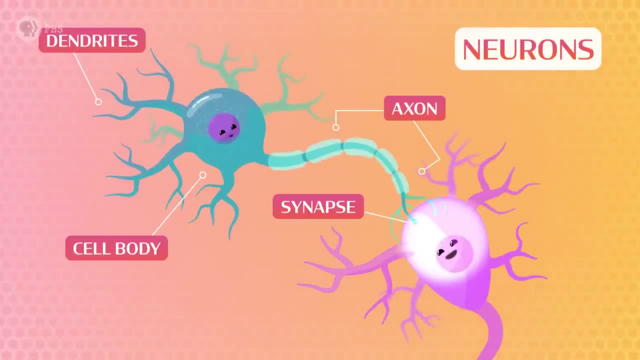 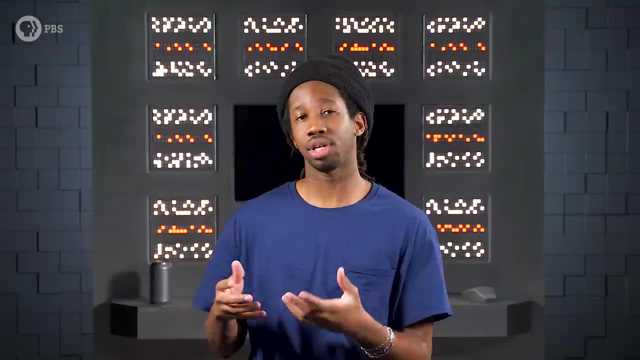 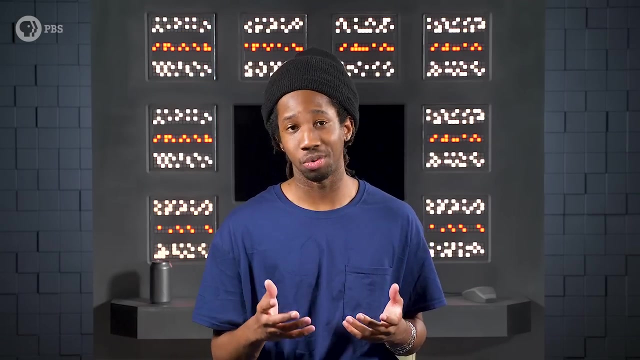 cell body builds up until a threshold is crossed. Then an electric signal shoots down the axon and is passed to another neuron Where everything repeats. The goal of early computer scientists wasn't to mimic a whole brain. Their goal was to create one artificial neuron that worked like a real one. To see how let's go to the 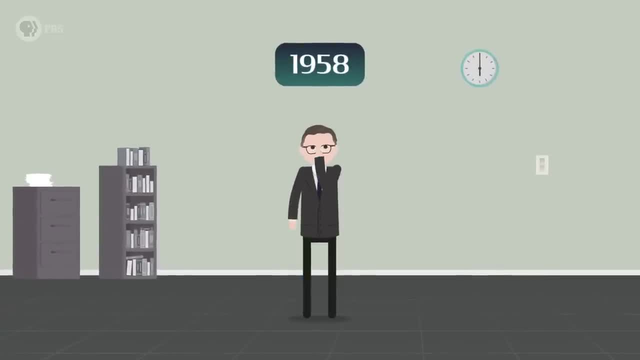 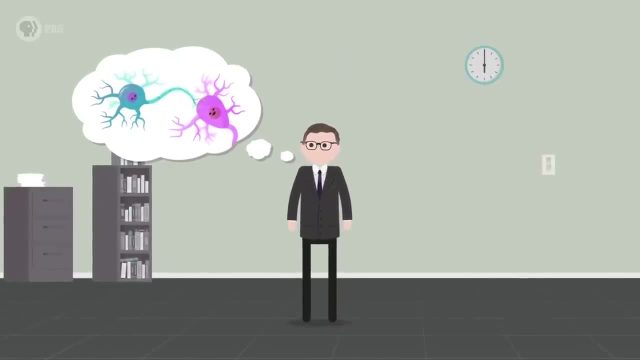 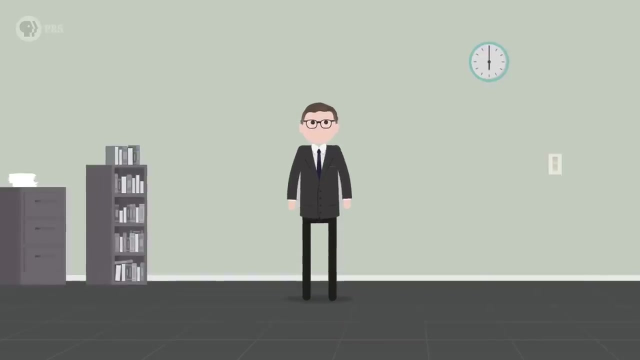 Thought Bubble In 1958, a psychologist named Frank Rosenblatt was inspired by the Dartmouth Conference and was determined to create an artificial neuron. His goal was to teach this AI to classify images as triangles or not triangles, with his supervision. That's what makes it supervised learning. The machine he built was about the size of 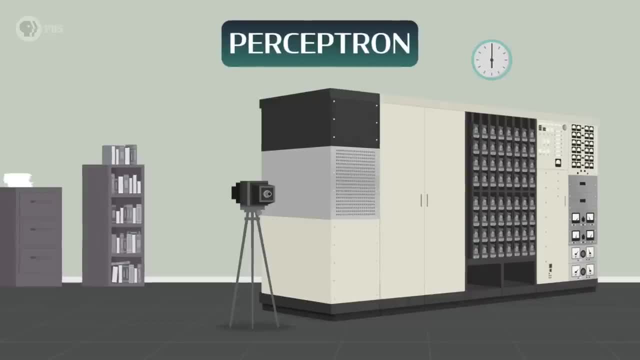 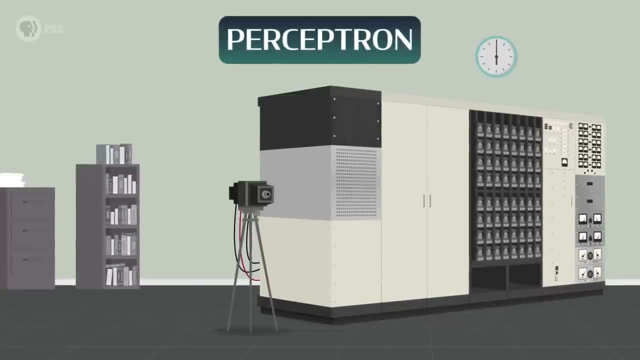 a grand piano and he called it the perceptron. Rosenblatt wired the perceptron to a 400-pixel camera, which was high-tech for the time but is about a billion times less powerful than the one on the back of your modern cell. 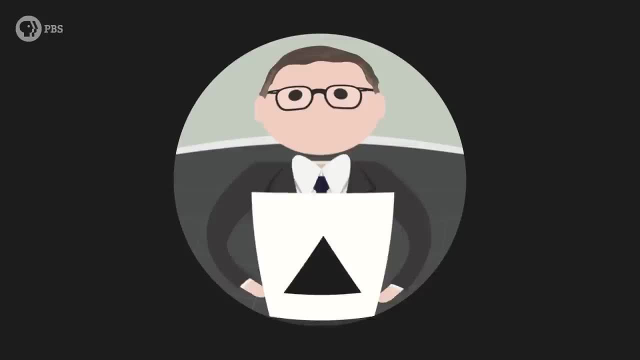 phone. He would show the camera a picture of a triangle or a not-triangle, like a circle, Depending on if the camera saw ink or paper. in each spot each pixel would send a different electric signal to the perceptron. Then the perceptron would add up all the signals that matched the signal to the perceptron. 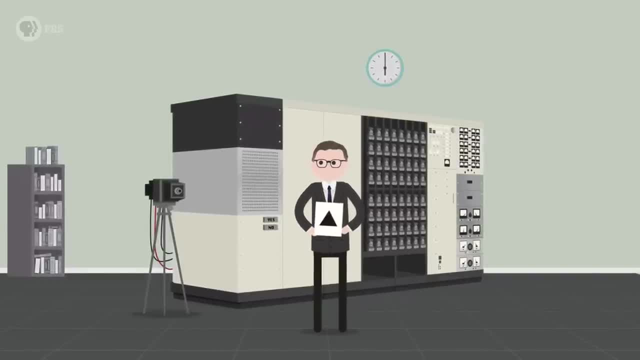 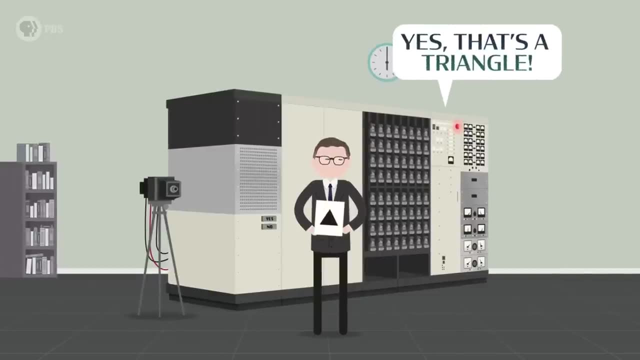 The perceptron would then send a different electric signal to the perceptron. Then the perceptron would match the triangle shape. If the total charge was above its threshold it would send an electric signal to turn on a light. That was artificial neuron speak for, yes, that's a triangle. 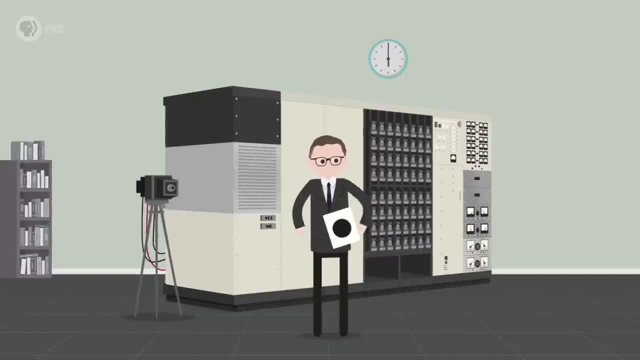 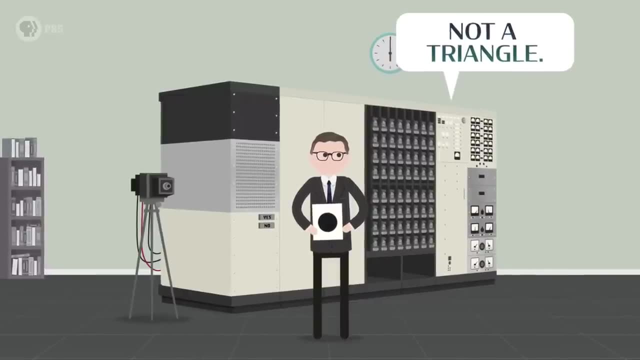 But if the electric charge was too weak to hit the threshold, it wouldn't do anything and the light wouldn't turn on. That meant not a triangle. At first the perceptron was basically making random guesses. So to train him with supervision, Rosenblatt used yes and no buttons. 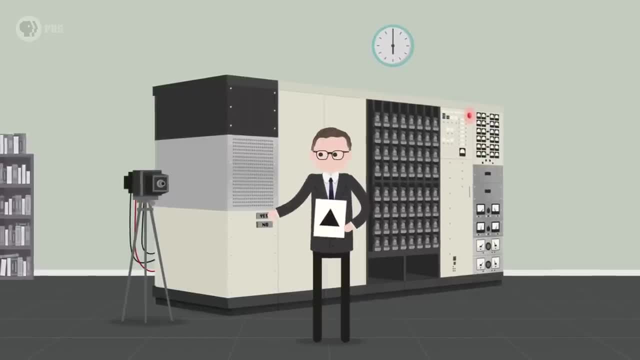 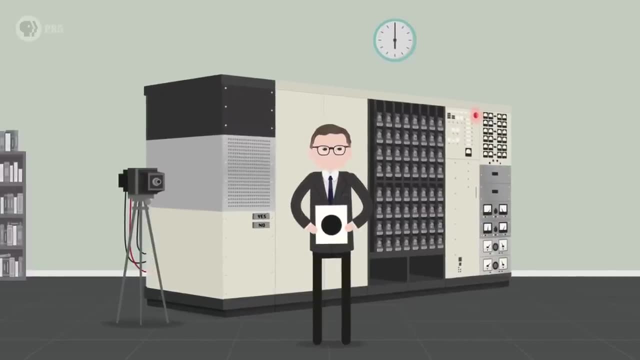 If the perceptron was correct, he would push the yes button And nothing would change. But if the perceptron was wrong, he would push the no button, which would set off a chain of events that adjusted how much electricity crossed the synapses and adjusted the machine's. 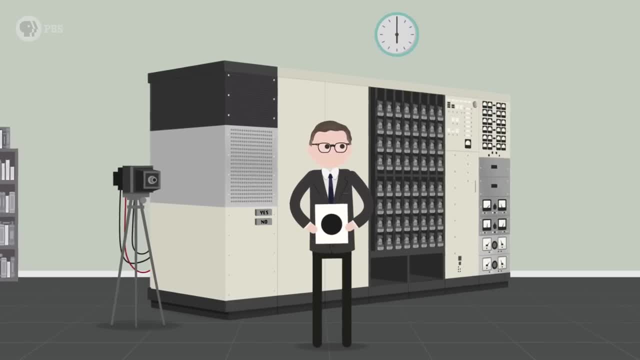 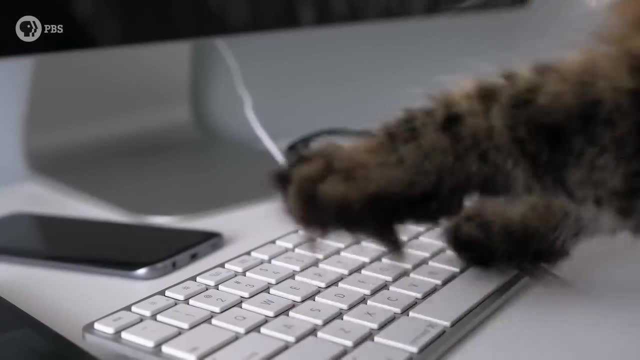 threshold levels, So it'd be more likely to get the answer correct next time. Thanks, Thought Bubble. Nowadays, rather than building huge machines with switches and lights, we can use modern computers to program AI to behave like neurons. The basic concepts are pretty much the same. 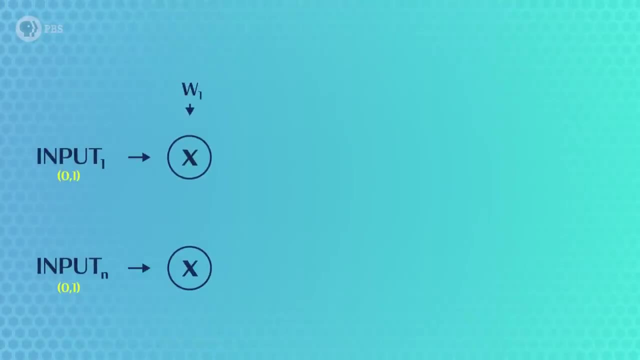 First, the artificial neuron receives energy. The artificial neuron receives energy. The artificial neuron receives inputs multiplied by different weights, which correspond to the strength of each signal In our brains. the electric signals between neurons are all the same size, but with computers 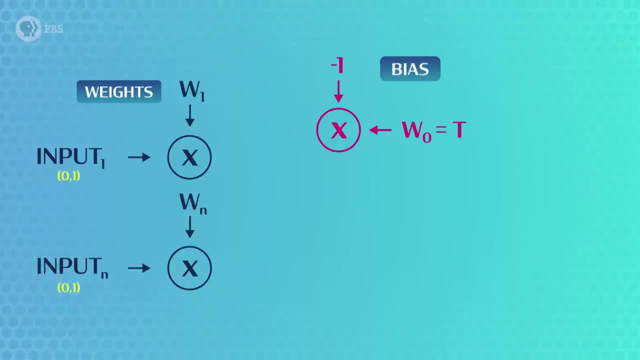 they can vary. The threshold is represented by a special weight, called the bias, which can be adjusted to raise or lower the neuron's eagerness to fire. So all the inputs are multiplied by their respective weights added together, and a mathematical function gets a result. 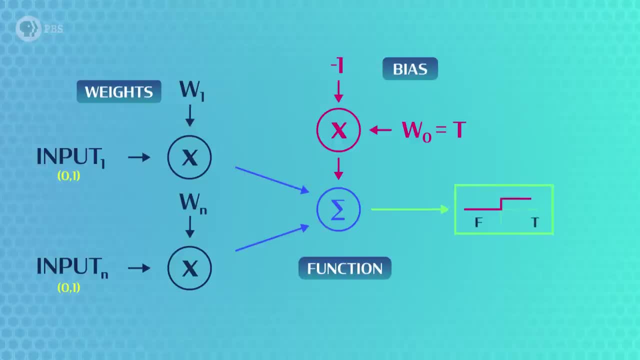 In the simplest AI systems, this function is called a step function- Step function, Which can only output a 0 or a 1.. If the sum is less than the bias, then the neuron will output a 0, which could indicate not triangle or something different, depending on the task. 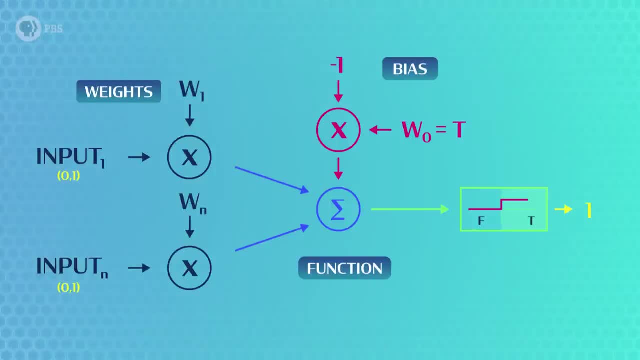 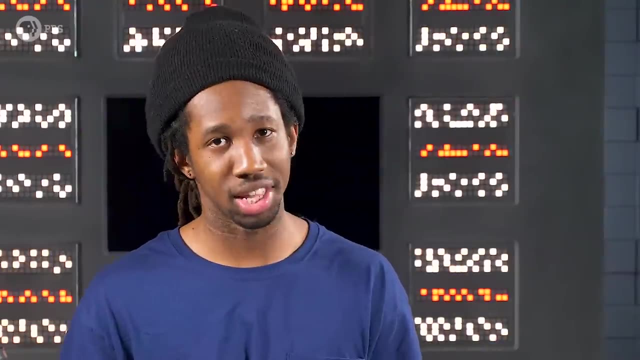 But if the sum is greater than the bias, then the neuron will output a 1,, which indicates the opposite result, And AI can be trained to make simple decisions about anything where you have enough data and supervised labels like triangles, junk mail, languages, movie genres or even similar. 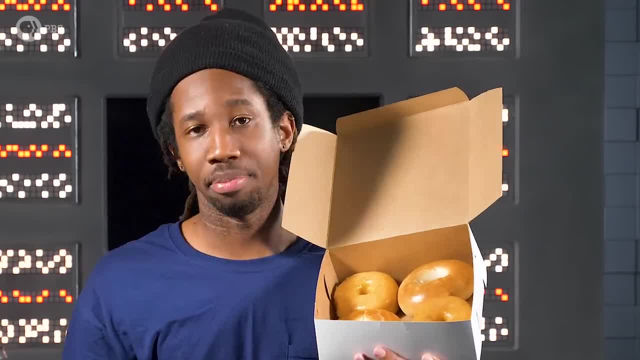 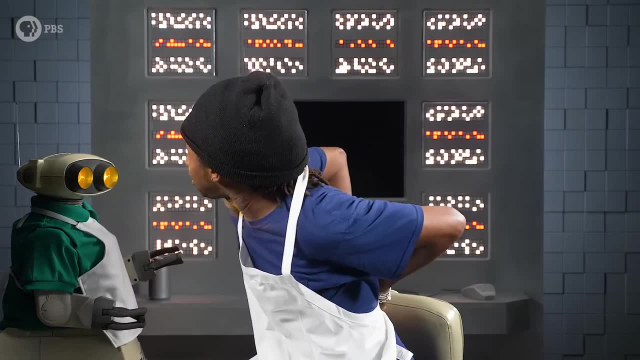 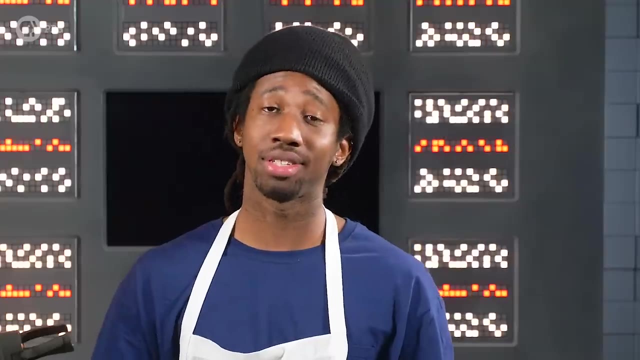 looking foods: doughnuts and bagels. Hey, John Green Bot, you want to learn how to sort some disgusting bagels from delicious doughnuts? John Green Bot still has to talk like a human program. Remember: we don't have generalized AI yet That. 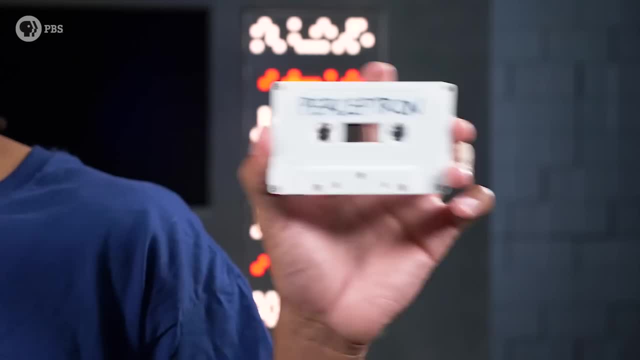 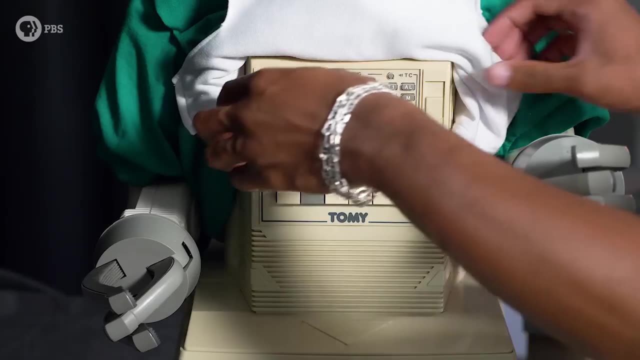 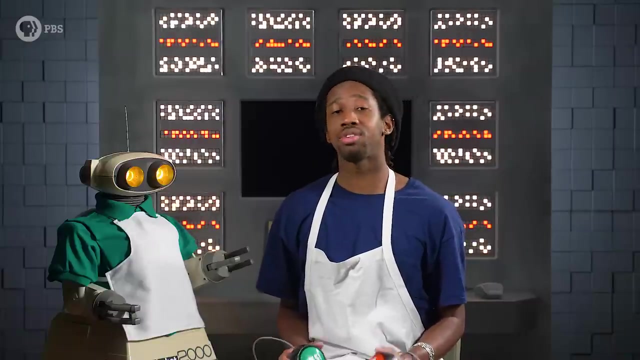 program is pretty limited, so I need to swap it out for the perception program. Now that John Green Bot is ready to learn, we'll measure the mass and diameter of some bagels and doughnuts and supervise him so he gets better at labeling them. 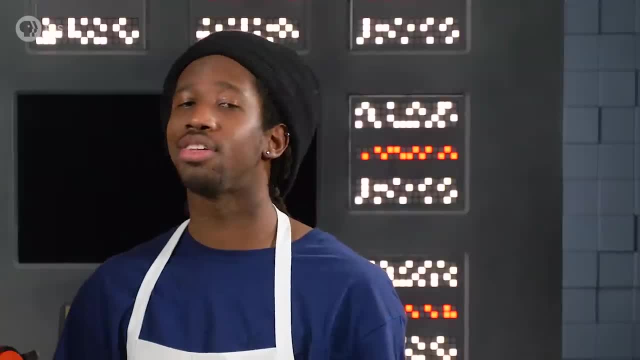 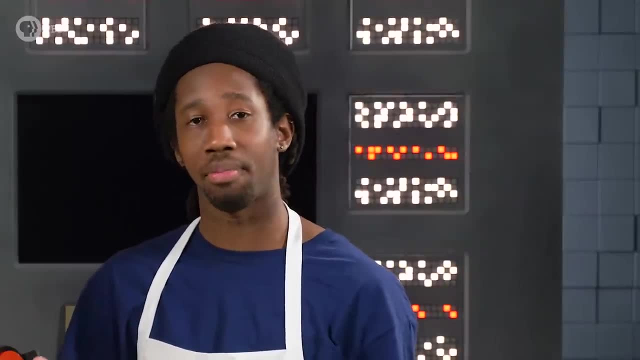 How about you hold on to these? for me Right now, he doesn't know anything about bagels or doughnuts or what their masses and diameters might be, so his program is initially using random weights for mass diameter and the bias to help make a decision. But 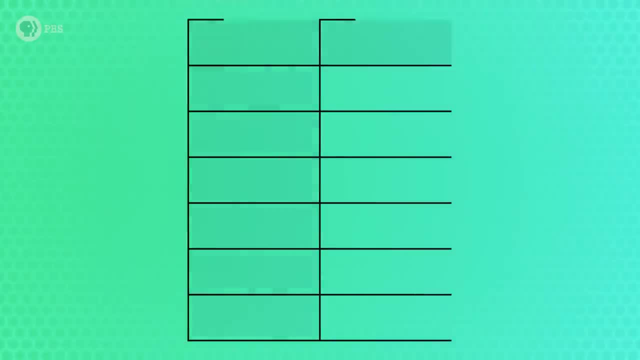 as he learns, those weights will be over. Now we can use different mathematical functions to account for how close or far an AI is from the correct decision, But we're going to keep it simple. John Green Bot's perception program is using a step function, So it's an either-or. 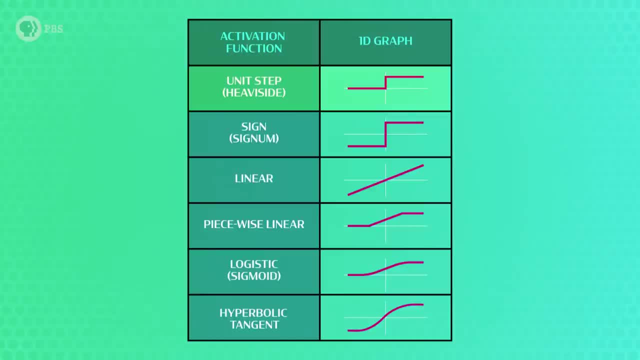 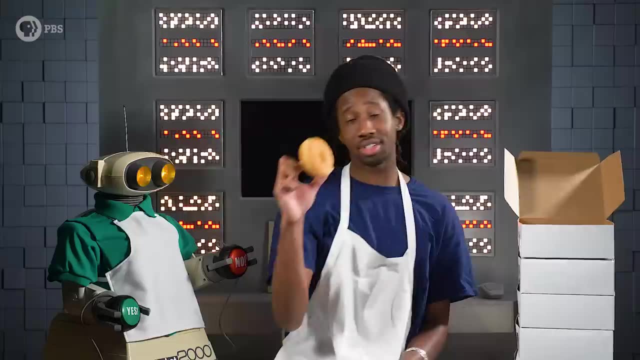 choice 0 or 1.. Bagel or doughnut- Completely right or completely wrong. Let's do this. This here is a mixed batch of bagels and doughnuts. This first item has a mass of 34 grams and a diameter of 7.8 centimeters. The 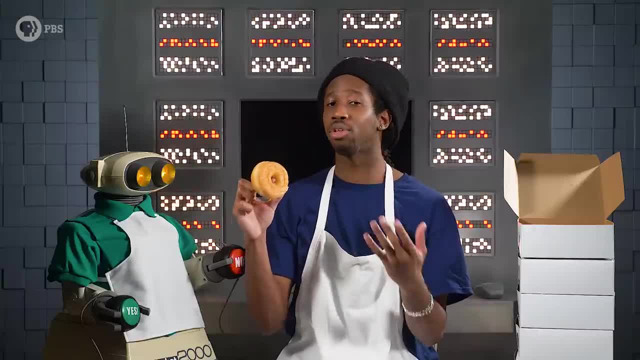 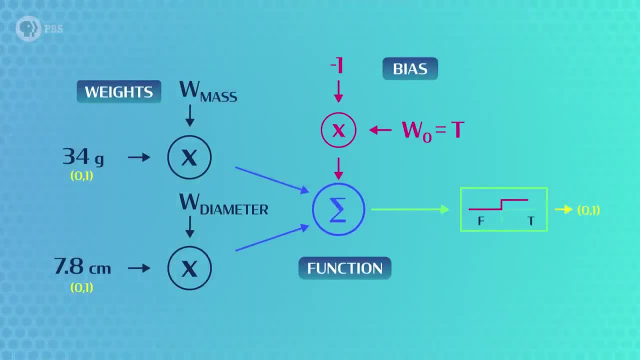 perception program actually uses a step function. The price is $10.10 for each bagel or doughnut. The perceptron takes these inputs, multiplies them by their respective weights, then adds them together If the sum is greater than the bias which, remember, is the threshold for the neuron. 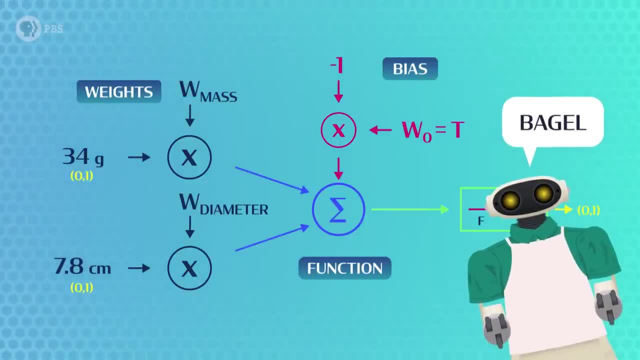 firing, John Greenbott will say bagel. So if it helps to think of it this way, the bias is like a bagel threshold: If the sum is less than the bias, it hasn't crossed the bagel threshold and John Greenbott 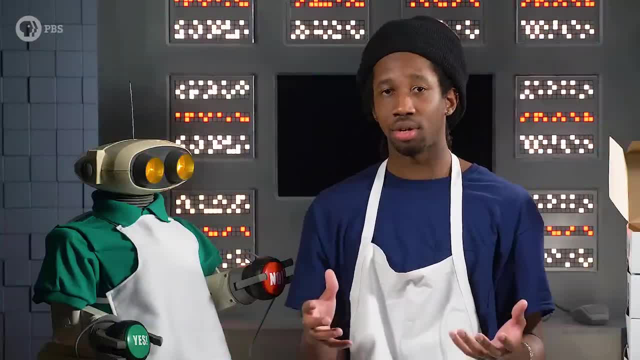 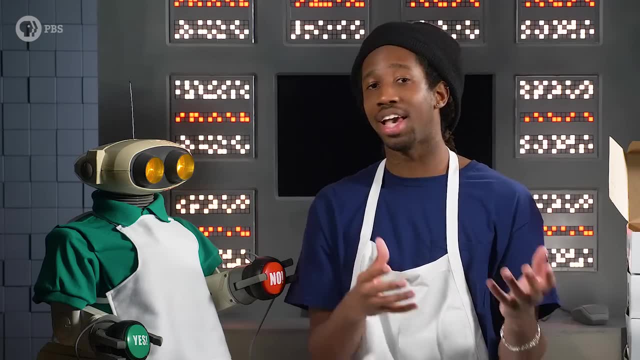 will say donut. All this math can be tricky to picture. So to visualize what's going on, we can think of John Greenbott's perceptron program as a graph with the mass on one axis and the diameter on the other. 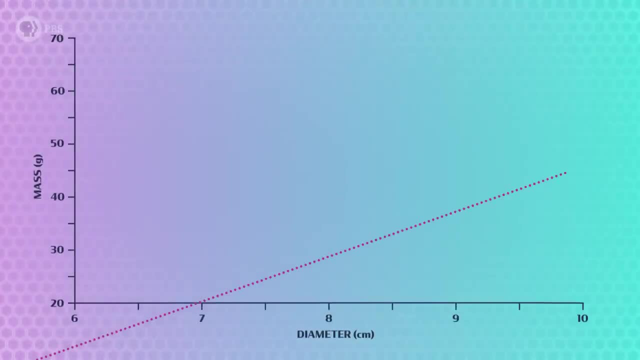 The weights and bias are used to calculate a line called a decision boundary on the graph which separates bagels from donuts, And if we represent this same donut as a data point, we'd graph it at 34 grams and 7.8. 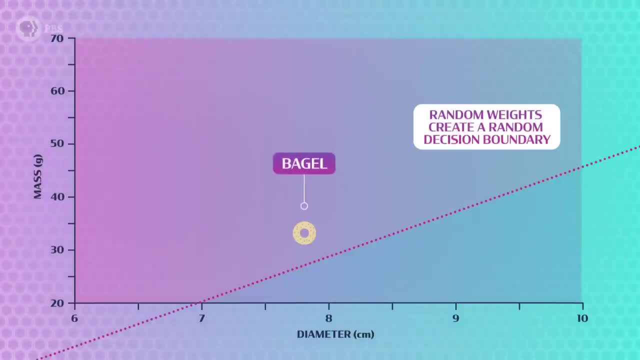 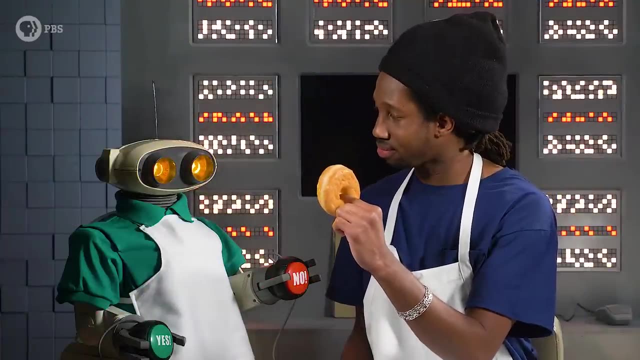 centimeters. This data point is above the decision boundary in the bagel zone. So all this means is, when I ask John Greenbott what this food is, he'll say bagel. And he got it wrong because this is a donut. 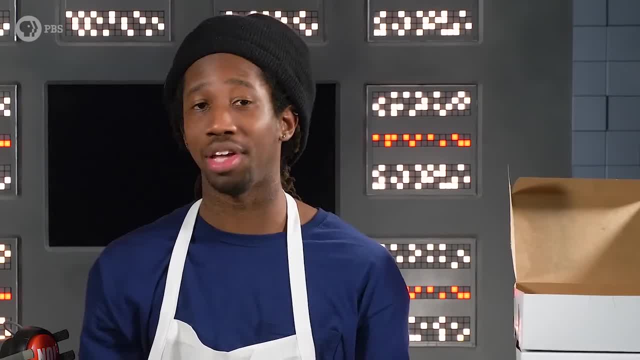 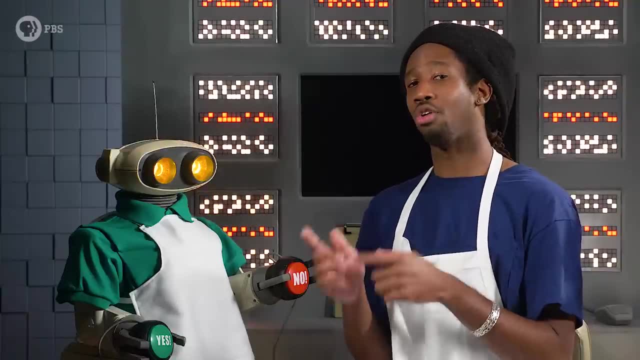 No big deal, though, With a brand new program. he's like a baby that made a random guess because he's using random weights right now, But we can help him learn by updating his weights. So we take an old weight and add a number calculated by an equation called the update. 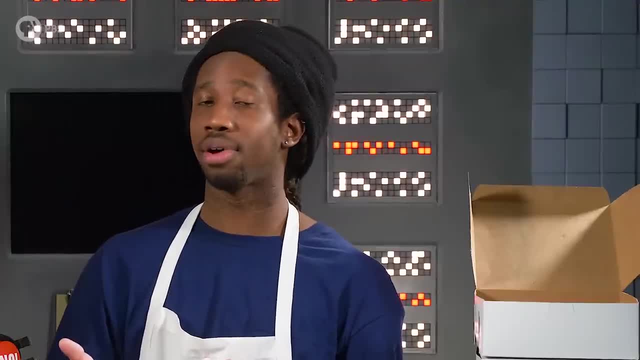 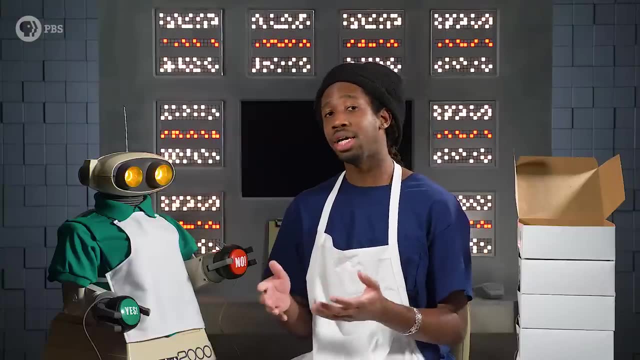 rule. We're going to keep this conceptual, but if you want more information about this equation, we've linked to a resource in the description. So let's get started, Because our perceptron can only be completely right or completely wrong. the update rule. 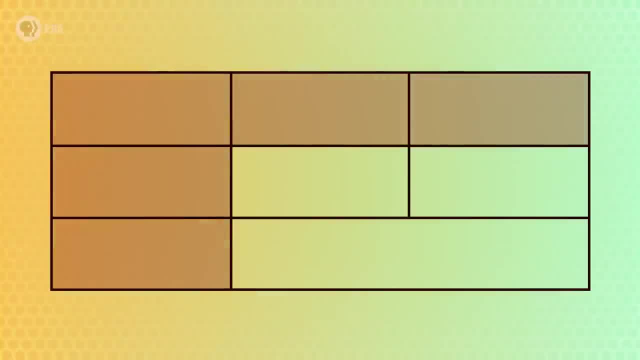 ends up being pretty simple. If John Greenbott made the right choice, like labeling a donut as a donut, the update rule works out to be zero, so he adds zero to the weight and the weight stays the same. But if John Greenbott made the wrong choice, like labeling a donut as a bagel, the update 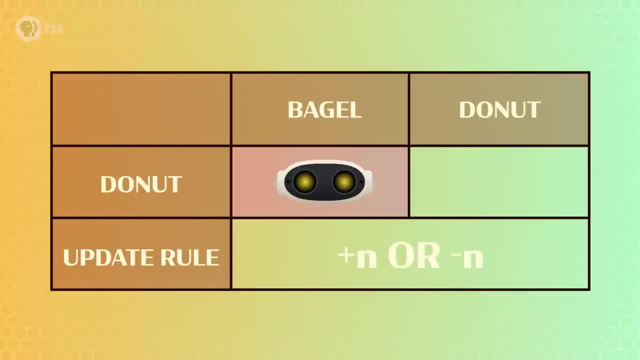 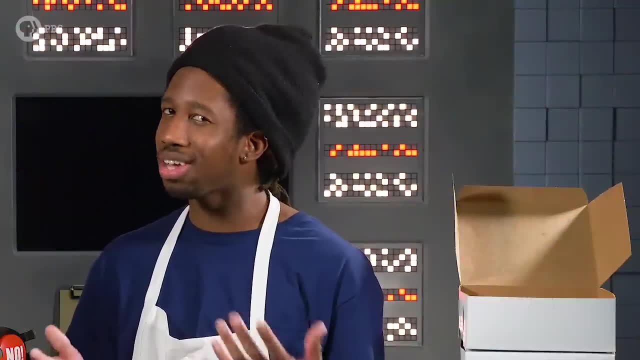 rule will have a value, a small positive or negative number. He'll add that value to the weight and the weight will change Conceptually. this means John Greenbott learns from failure, and he's going to have to learn from failure but not from success. 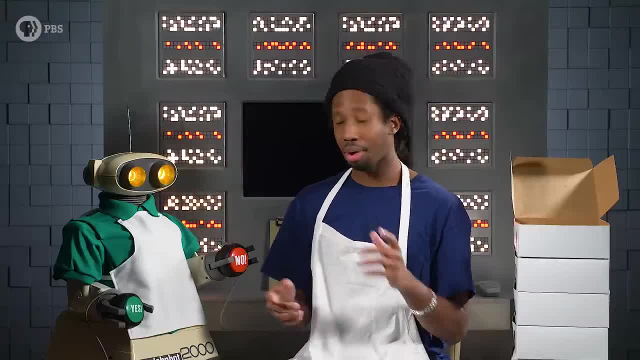 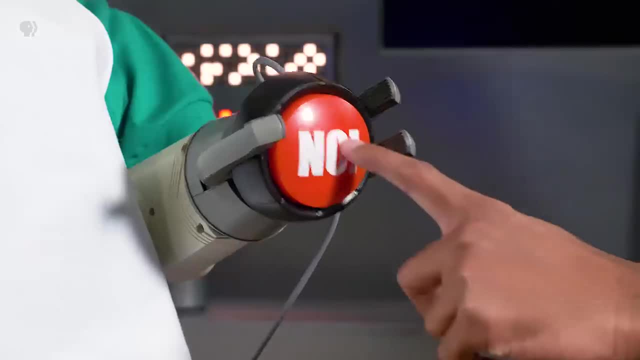 So he called this donut a bagel and got the label wrong By pressing this no button. I'm supervising his learning and letting him know that he made the wrong choice. So his weights update. If we look back at the graph, we can see that when the weights update, the decision boundary. 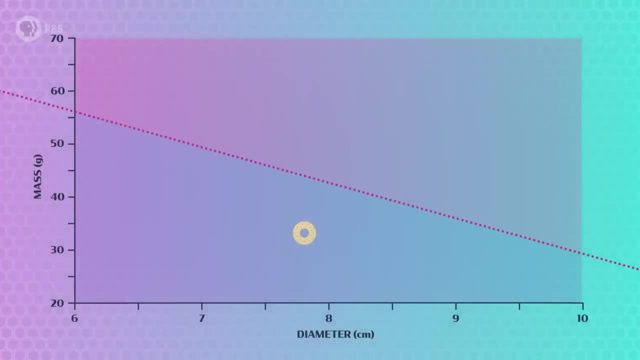 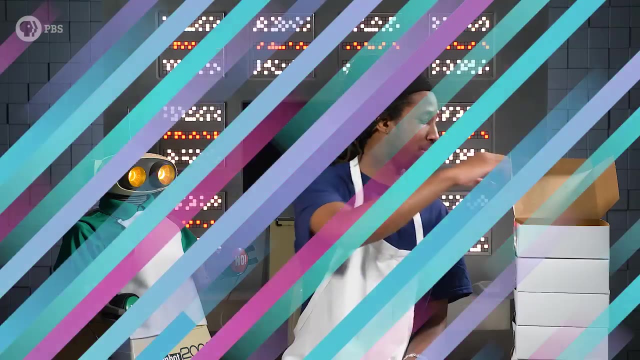 changes. That data point we added is now below the line in the donut zone. Now his perceptron will classify another item with this mass and diameter as a donut. This next item has a mass of 28.5.. It's 26 grams and a diameter of 6.1 centimeters. 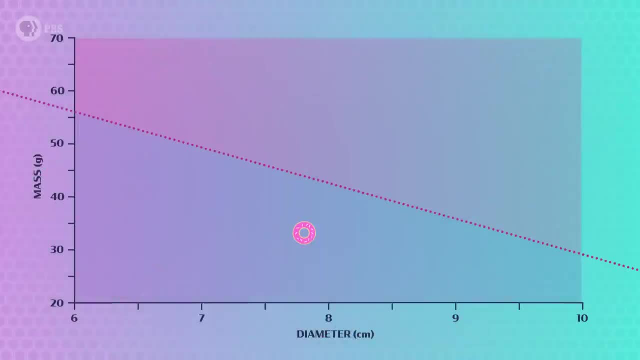 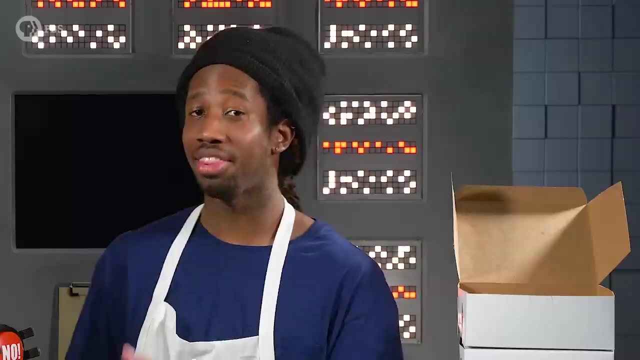 What do you think, John Greenbott? He got it right When he took those inputs and did the same calculation. the sum was less than the bias. That data point appeared below the decision boundary in the donut zone, And so I'm going to push the yes button. 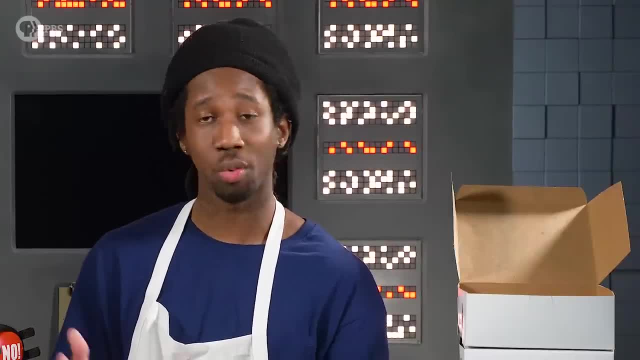 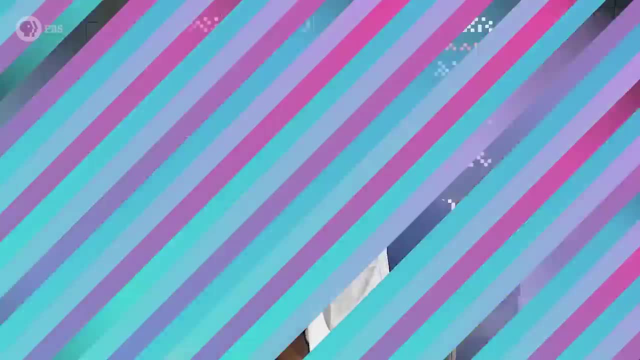 In this case, the update rule equation works out to be zero, So the weights are the same and so does the decision boundary. Now we do this 48 more times. I'm going to do this 48 more times to train his perceptron. 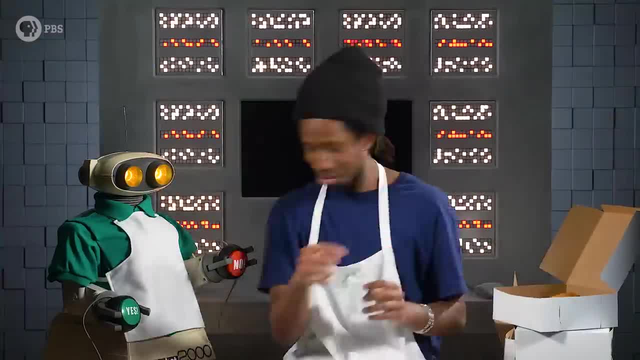 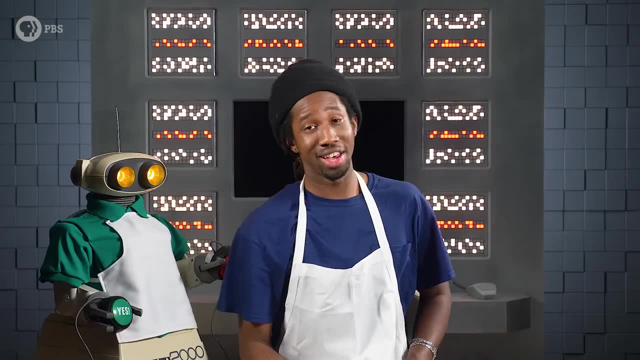 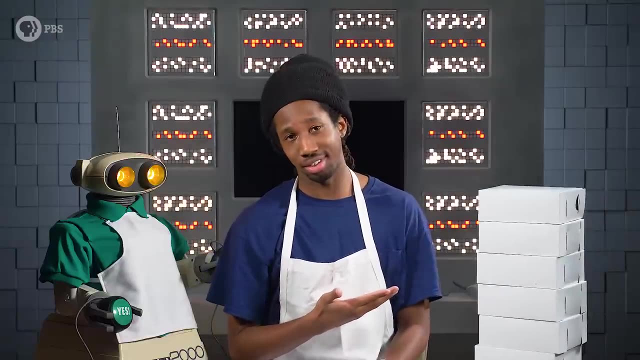 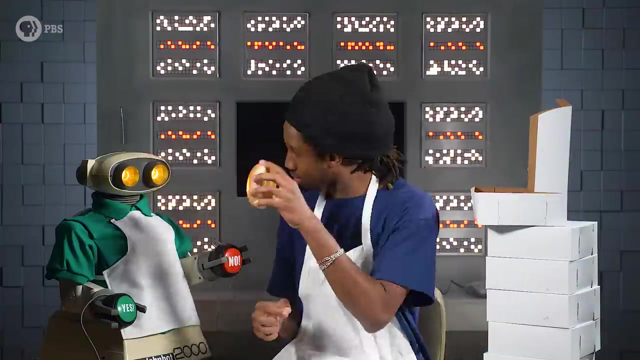 After we're done training John Greenbott's perceptron, we have to test it on new data to see how well he's learned. So I got a hundred new bagels and donuts for him to classify. Woah, Woah. 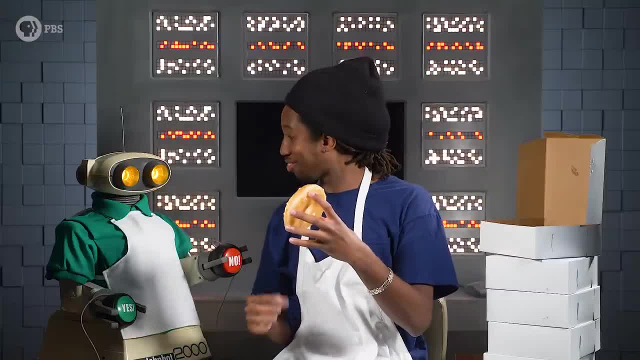 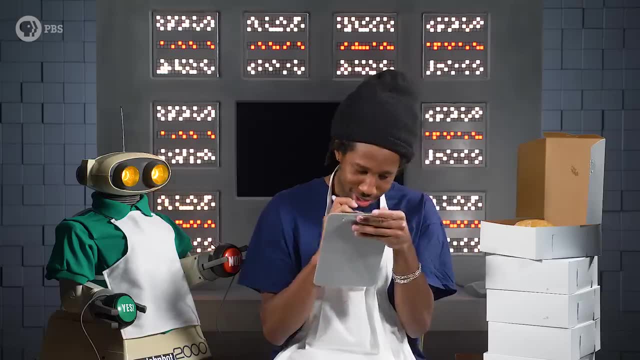 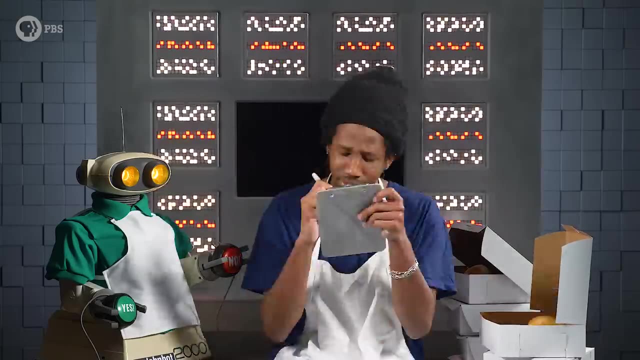 This is a big what? What is this Bagel? Alright, Alright, Just let me write that down. Write it down on your end. Sure, Okay, Alright. So overall, he's classified 25 donuts and 75 bagels. 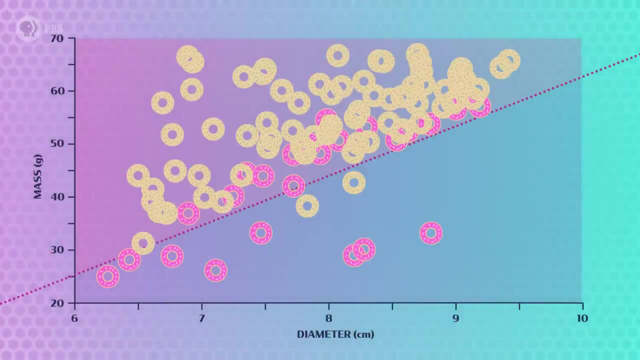 We can visualize the results on a graph with the decision boundary like this: So he's got a lot of doughnuts. He's got a lot of bagels. He's got a lot of donuts, He's got a lot of doughnuts. 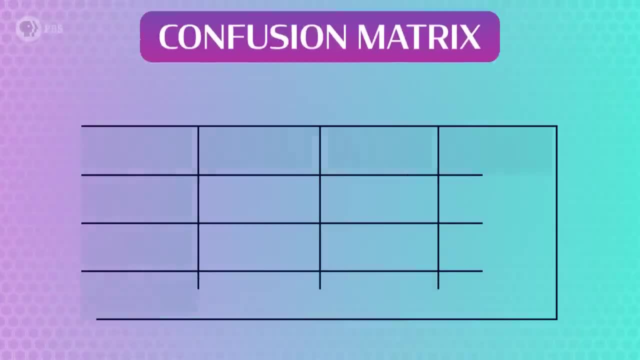 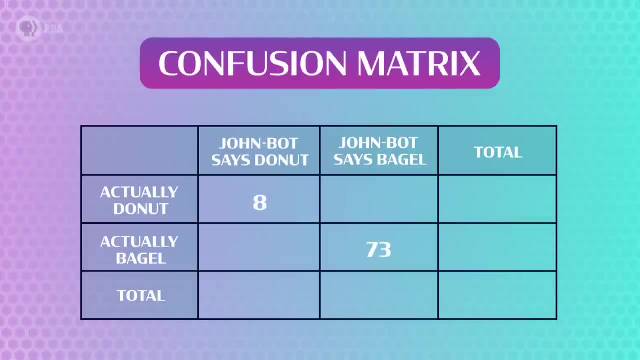 like this, But we can also put the results in a table called a confusion matrix, because it tells us where John Greenbot was confused. He got 8 donuts correct and 73 bagels correct, But he said that a bagel was a donut twice and that a donut was a bagel 17 times. 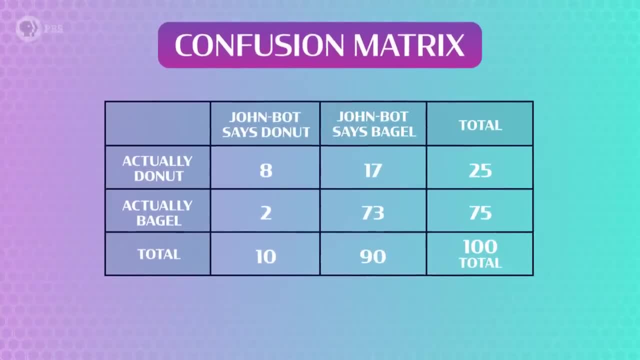 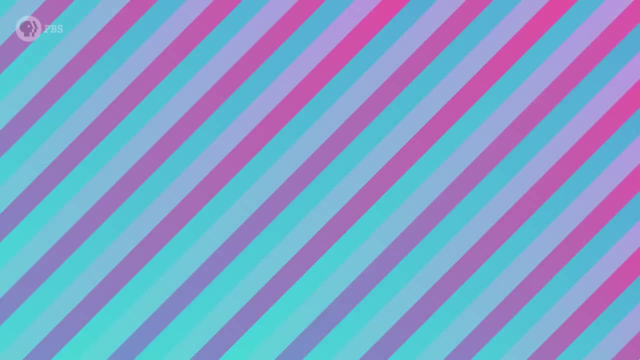 Using these numbers, we can calculate his overall accuracy by adding together what he got right, which were 8 donuts and 73 bagels, and dividing by the total 100 to get 81%. But to really understand what's wrong we need to take a look at his precision and 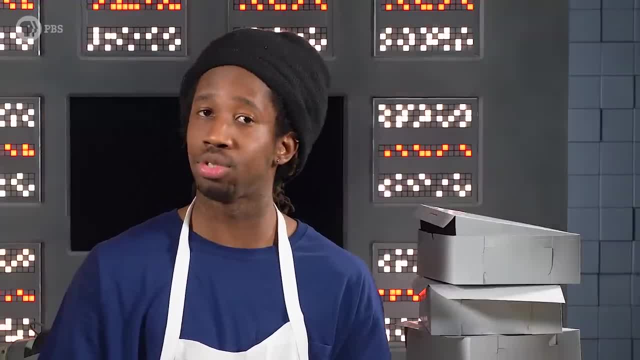 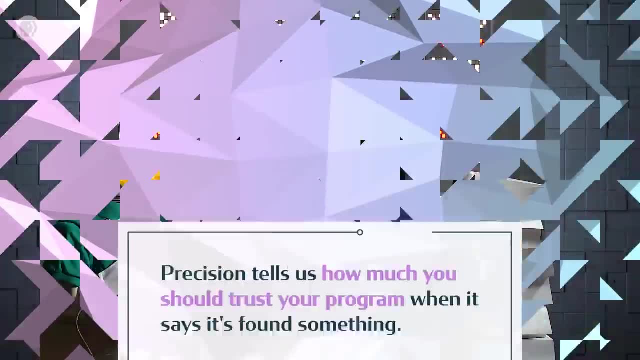 his recall. We can calculate these percentages for both foods, but we'll focus on donuts right now. Precision tells us how much you should trust your program when it says it's found something. If John Greenbot tells me something's a donut, I'm expecting to eat a donut. 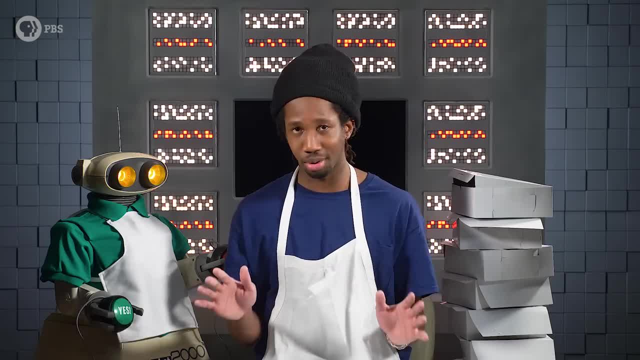 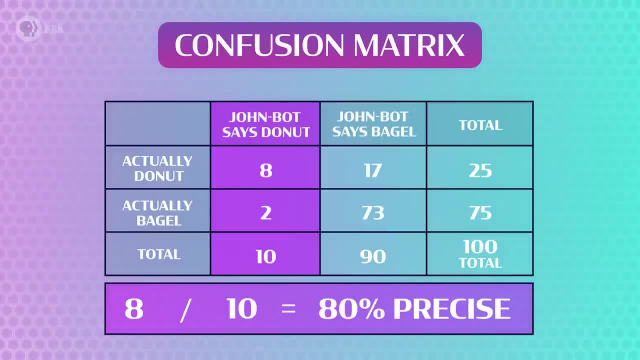 I don't want to bite into a bagel because that would be a gross surprise. Of the 10 items he said were donuts, 8 were actually donuts. so he was 80% precise And I can be 80% sure he's only handing me donuts when he says he is. 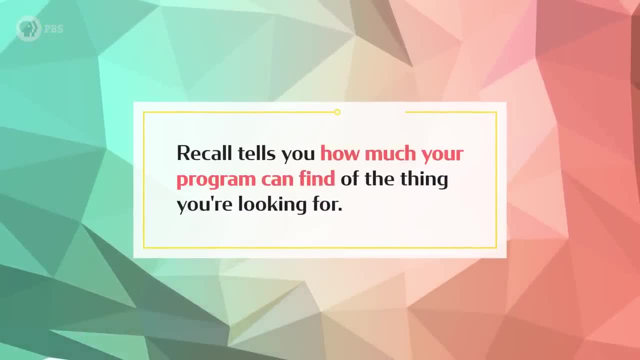 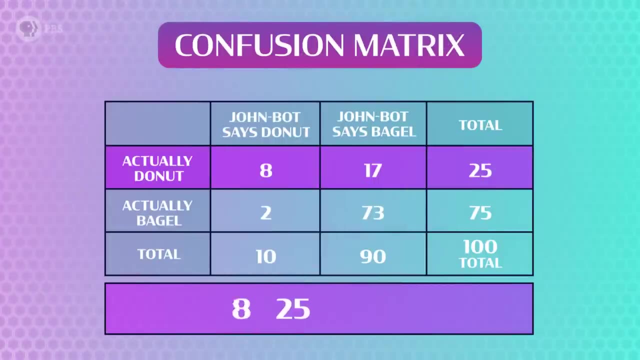 Recall tells you how much your program can find of the thing you're looking for. I'm really hungry, so I want as many donuts as possible, But of the 25 items that were donuts, he correctly labeled 8 of them. 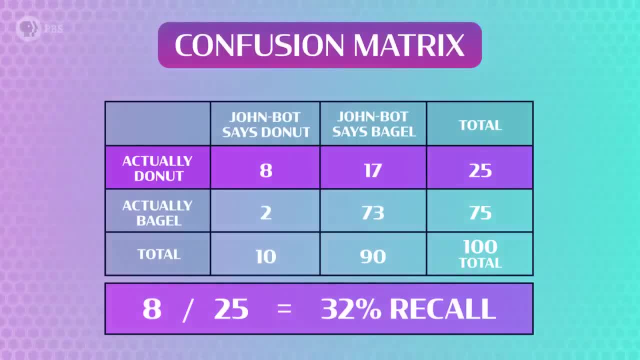 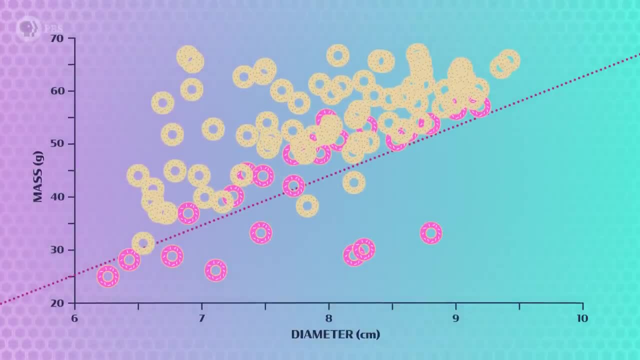 So his recall is just 32% and he just handed me 32% of all the donuts. The precision and recall depend on the criteria John Greenbot is using to make a decision- Diameter and mass- And, as you can see from this graph, John Greenbot is using the same criteria as John Greenbot. 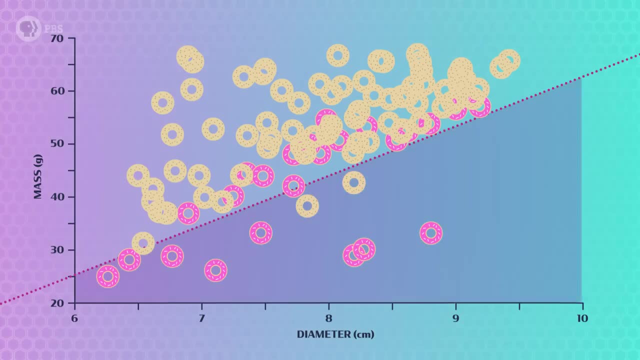 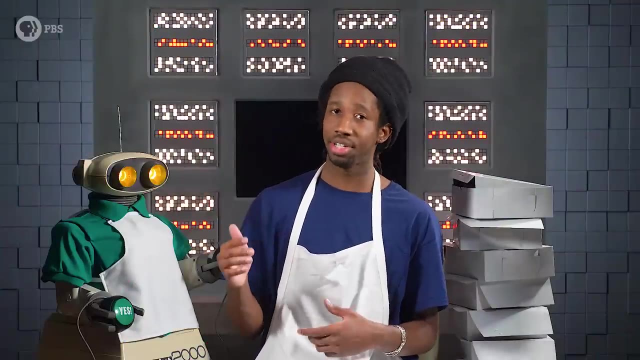 is using to make a decision In his graph. he thinks that donuts generally have smaller diameters and masses than bagels. They're small, fluffy treats. So when it comes to classifying donuts he has a high precision, because if he says something's.